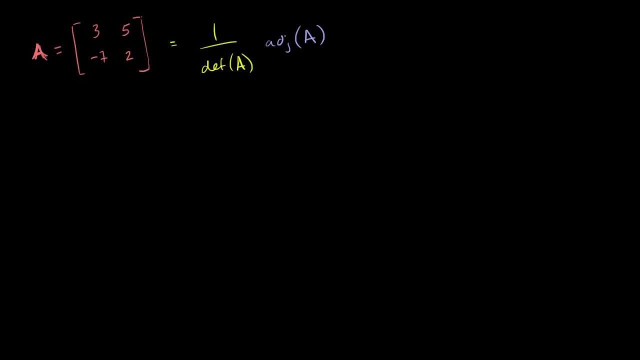 So first let's think about what the determinant of this matrix is. Well, we've seen this before. We just look along the two diagonals. It's 3 times 2 minus negative, 7 times 5.. So this is going to be equal to 1 over 3 times 2 minus negative. 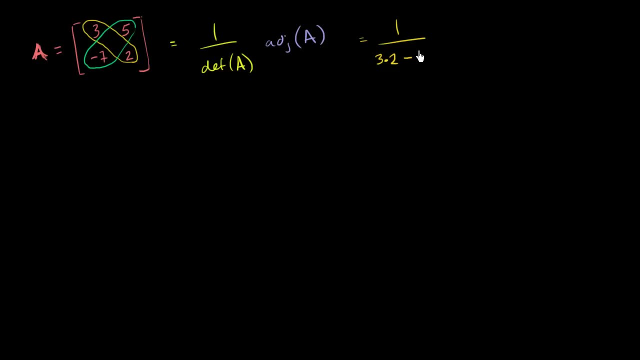 7. So minus negative 7 times 5.. And then the adjugate of a, and here I'm really just teaching you the mechanics of it, And it's a little unfortunate that in a typical Algebra 2 class you kind of have to just go into the mechanics of it. 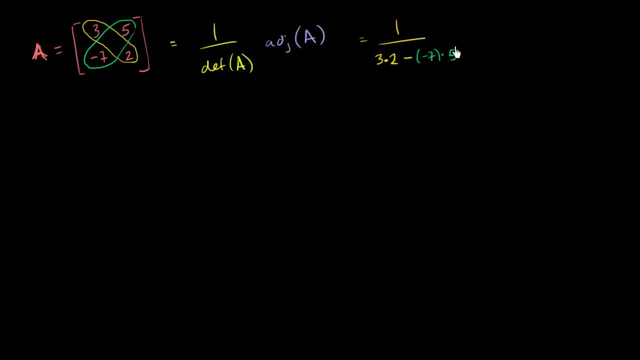 But at least this will get us to where we need to go. So the adjugate of a: you literally just need to swap the two elements on this diagonal. So put the 2 where the 3 is and the 3 where the 2 is. 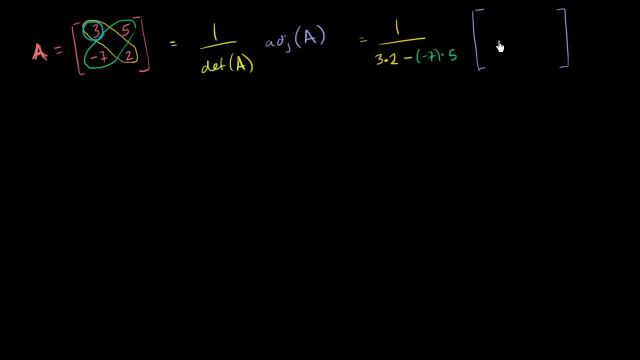 So this element right over here, this 3 will go right over there, This 2 will go right over here, And then these two elements. you just take the negative of them. So the negative. let me do a new color. Actually I'm running out of colors. 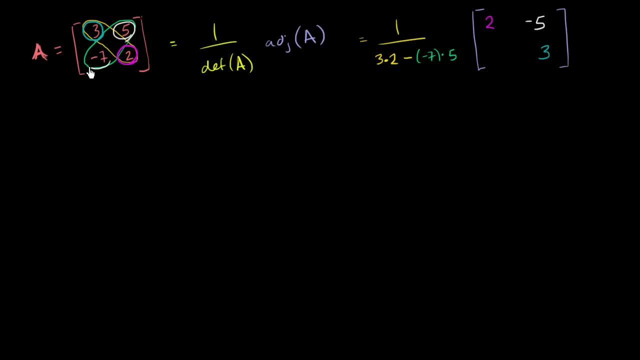 The negative of that is negative: 5.. The negative: The negative of that is positive: 7.. So we are left with: this is going to be equal to: 1 over 3 times 2 is 6.. Negative: 7 times 5 is negative: 35.. 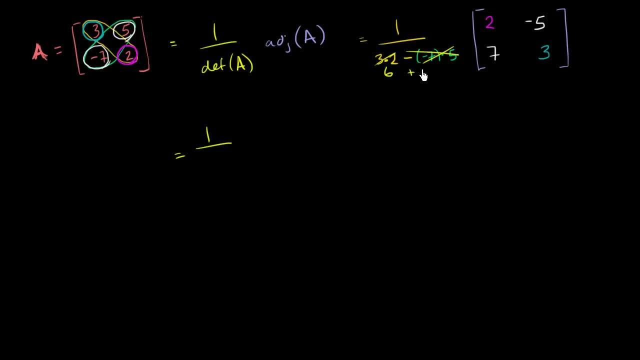 But then we have this positive over here, So this whole thing becomes plus 35. So 6 plus 35 is 41. So the determinant of our matrix is 41. We're going to take 1 over the determinant and multiply it times our adjugate, times 2,, negative 5,. 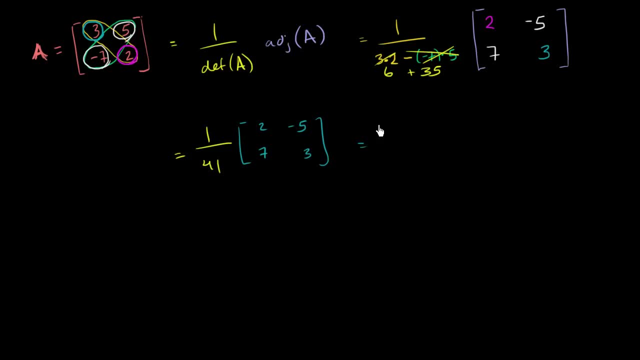 7, and 3.. So we get. so this is the drum roll part: 2 over 41.. Negative: 5 over 41.. I'm just multiplying each of these elements times 1 over 41.. 7 over 41 and 3 over 41. And we are done.